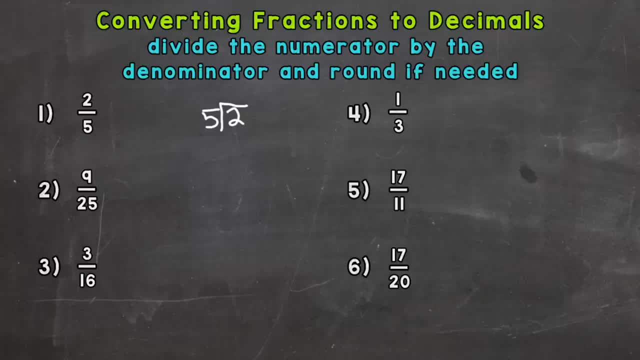 group of five out of that two. So we need to extend our division problem by putting a decimal and a zero, So now we can think of that as 20.. Bring our decimal straight up. How many whole groups of five can we divide by? 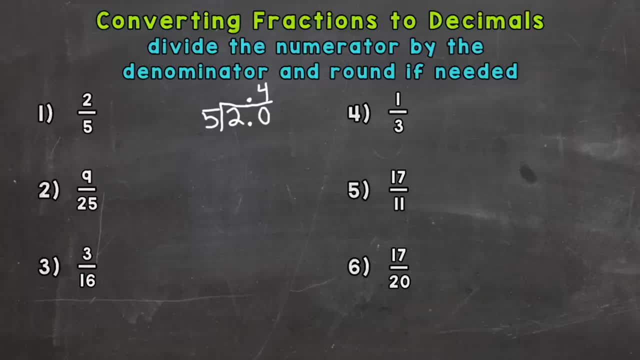 We pull out of 20.. Well, four, Four times five is 20.. Subtract and we get a zero And that tells us we are done. So two-fifths is equal to four-tenths. Number two, nine-twenty-fifths. 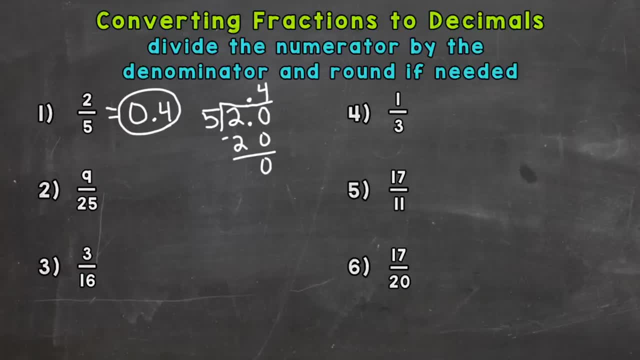 I'll do this one by hand as well. So nine divided by 25.. So we need to extend our division problem with a decimal and a zero, because we can't do nine divided by 25 and get a whole number. We can't pull a group of 25 out of nine. So now we think of 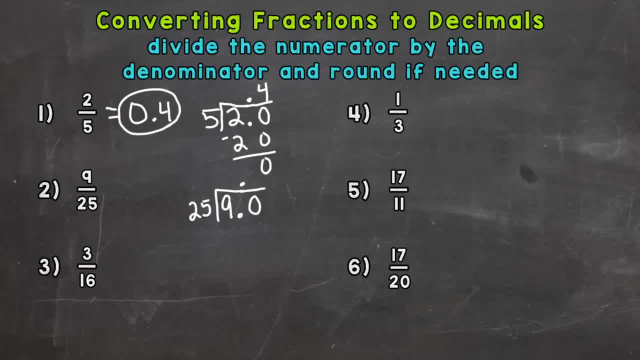 this as 90. How many whole groups of 25 out of 90?? Well, three, Three times 25 is 75. Subtract and we get 15.. So we did not get a zero right away like number one, So we can extend this division. 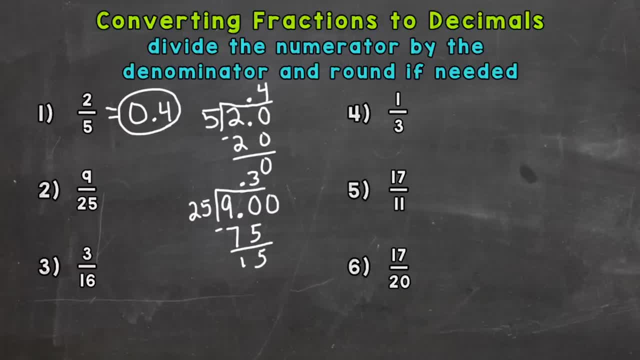 problem by putting another zero on the end. A zero to the right of a decimal doesn't change the value, So we're not changing the problem at all. Now we can bring that zero down and we have 150 divided by 25. And we can pull six whole 25 out of 90. So now we need to 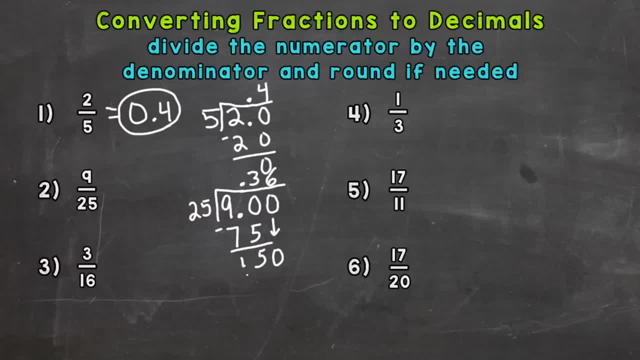 have 150.. Six times 25 is 150. And we get that clean cut zero, So we do not need to go any further. We are done. And that problem kind of ran into the top problem there. But our answer is 36-hundredths. 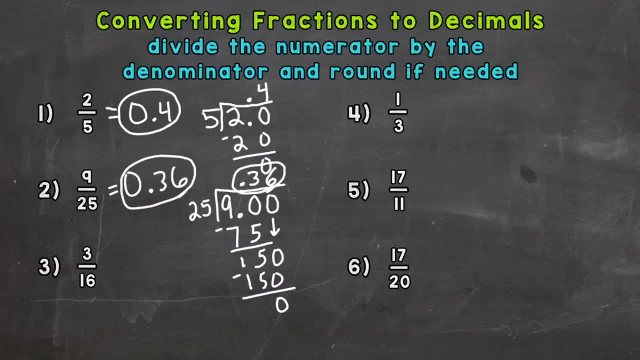 So nine-twenty-fifths is equal to 36-hundredths. Let's take a look at number three. Now number three: if we were to plug in three divided by 16 into a calculator, we would get the following decimal, And it goes to the ten-thousandths. So it's typical to either round a decimal 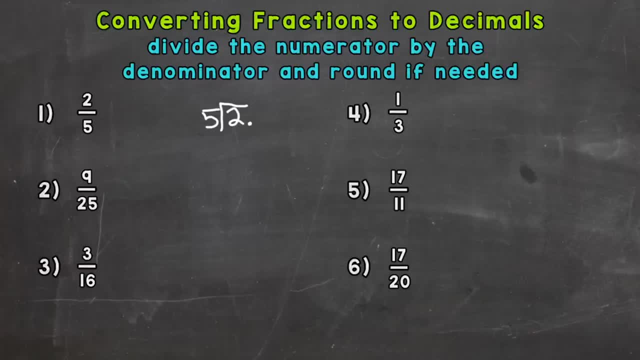 So we need to extend our division problem by putting a decimal and a zero. So now we can think of that as 20.. Bring our decimal straight up. How many whole groups of five can we pull out of 20?? Well, four. 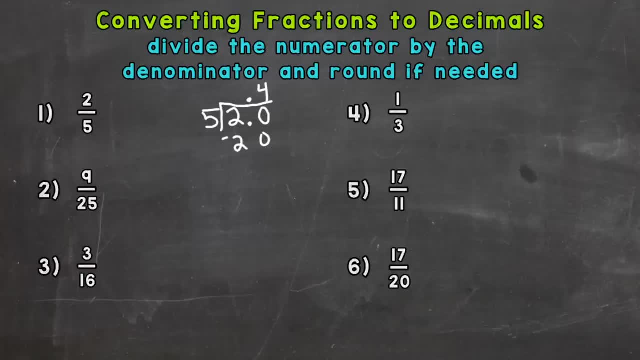 Four times five is 20.. Subtract and we get a zero and that tells us we are done. So two-fifths is equal to four-tenths. Number two: nine, twenty-fifths. I'll do this one by hand as well. 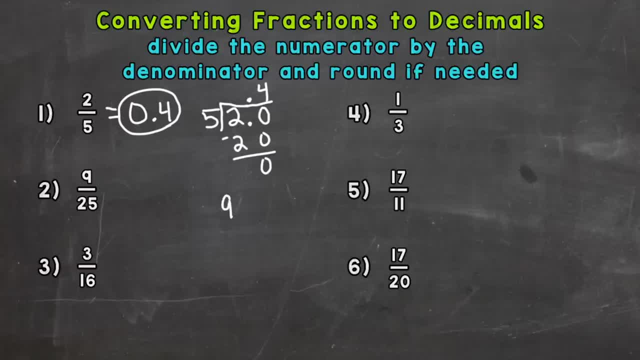 So nine, Nine divided by twenty-five. So we need to extend our division problem with a decimal and a zero, because we can't do nine divided by twenty-five and get a whole number. We can't pull a group of twenty-five out of nine. 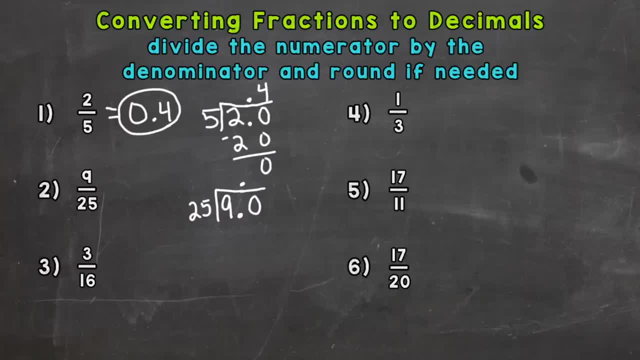 So now we think of this as ninety, How many whole groups of twenty-five out of ninety? Well, three, Three times twenty-five is seventy-five Subtract and we get fifteen. So we did not get a zero right away like number one. 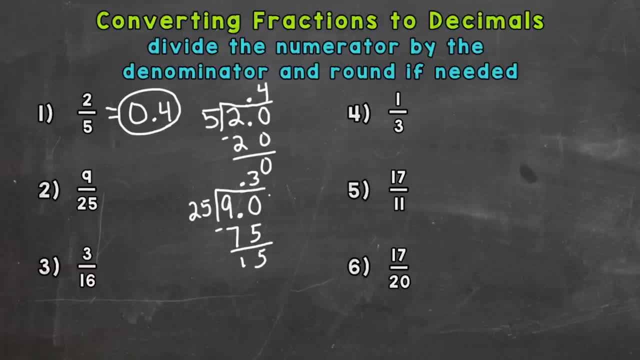 So we can extend this division problem by putting another zero on the end. A zero to the right of a decimal doesn't change the value, so we're not changing the problem at all. Now we can bring that zero down and we have one hundred fifty divided by twenty-five. 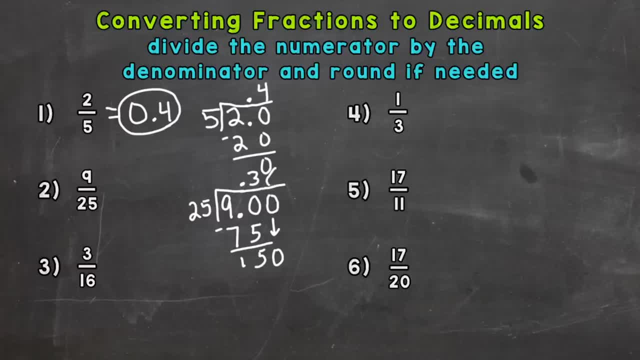 And we can pull sixty-five, six, whole 25 out of 150.. Six times 25 is 150. And we get that clean cut zero. So we do not need to go any further. We are done. And that problem kind of ran into the top problem there. But our answer: 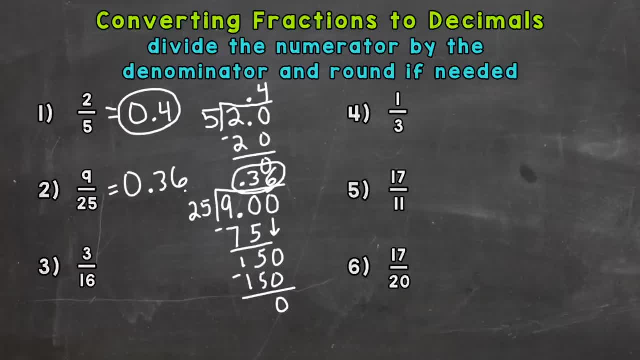 is 36 hundredths. So nine twenty-fifths is equal to 36 hundredths. Let's take a look at number three. Now number three: if we were to plug in three over three, divided by 16, into a calculator, we would get the following decimal, And it goes to the ten thousandths. 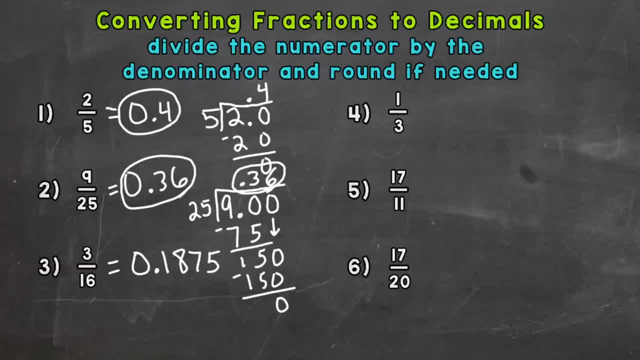 So we get the following decimal And it goes to the ten thousandths. So we get the following decimal And it goes to the ten thousandths. So it's typical to either round a decimal to the thousandths or hundredths. So we're going to round. 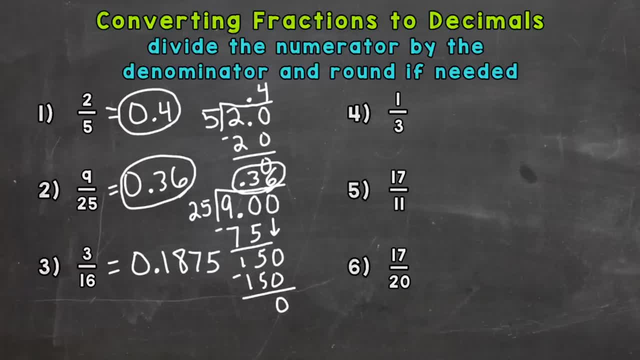 to the thousandths in this video. So we would take a look at what's in the thousandths. Look next door. That five says round up. We are closer to 188 thousandths, So our rounded answer would be 188 thousandths. 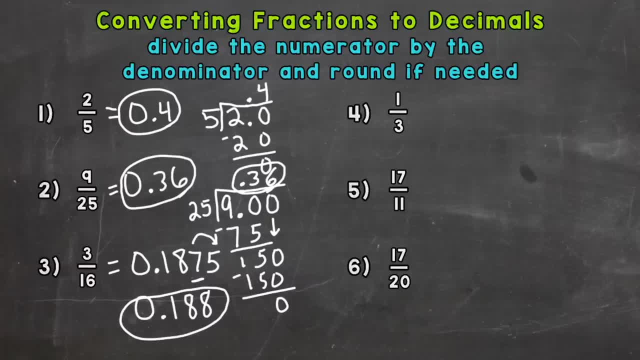 We are closer to 188 thousandths, So our rounded answer would be 188 thousandths. So our rounded answer would be 203 thousandths, And that makes us 6,000.. So that rounding step depends on what you are doing with the problem. 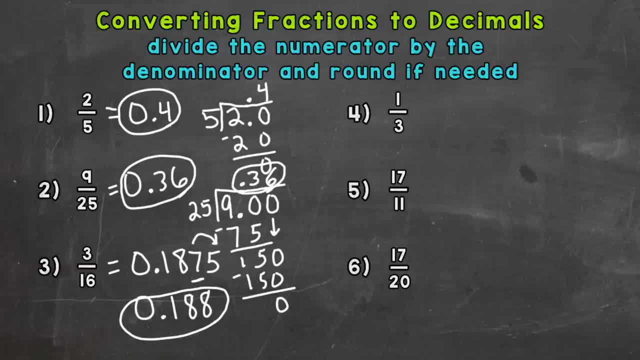 Maybe you wouldn't round that decimal. depending on the situation And as we'll see with the number four and five, we can have decimals that are much longer than just to the ten thousandths place. We can have decimals that are much longer than just to the ten thousandths place. 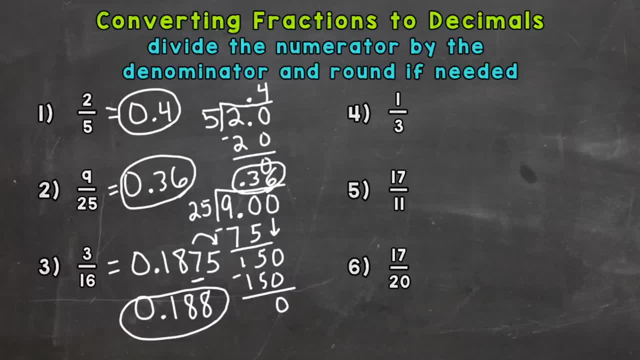 So, speaking in a number four, here we have one over three or one third, And I'm going to show you this by hand and hopefully- And I'm going to show you this by hand, and hopefully you'll notice a pattern as I start doing this- one, So 1 divided by 3.. So, again, this is just like. 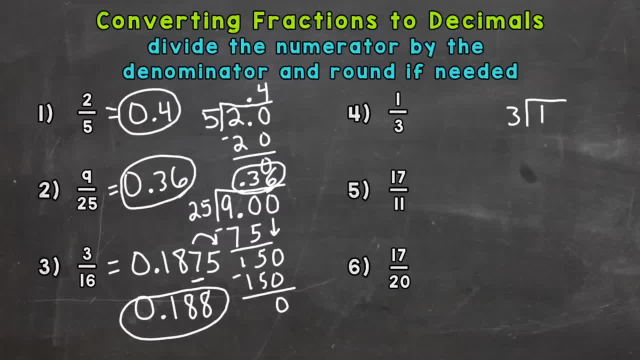 number 1 and 2, where we wrote them out. We can't pull a whole 3 out of that 1, so we extend with a decimal and a 0.. Bring that decimal straight up, So we look at it as a 10.. So how many whole 3's? 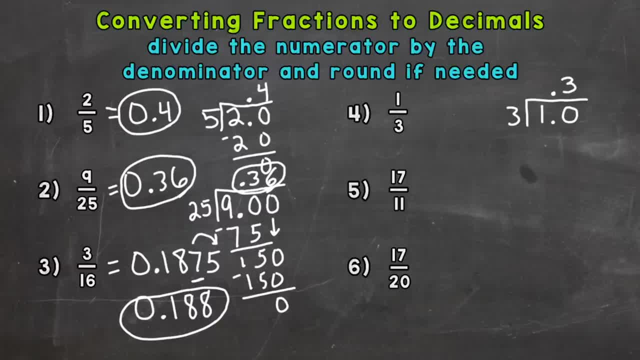 can we pull out of 10?? Well, 3.. That gets us to 9.. 3 times 3 is 9.. Subtract, we get 1.. Remember, we want that clean. cut 0 to tell us that we are done, So we need to add another 0. Drop it, So we have. 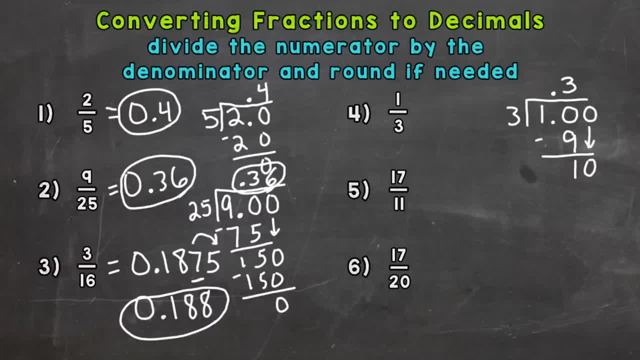 another 10.. How many whole 3's out of 10? Well, 3.. 3 times 3 is 9.. And our pattern is going to start here: Subtract, Add another 0 and drop it, So we have another 10.. 3, 3's out of 10.. 3 times 3 is 9.. Subtract A 1.. 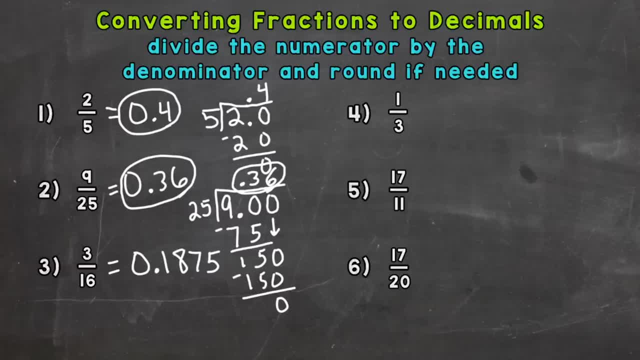 to the thousandths or hundredths. So we're going to round to the thousandths in this video. So we would take a look at what's in the thousandths. Look next door. That five says: round up, We are closer to one-hundred-eighty-eight thousandths. 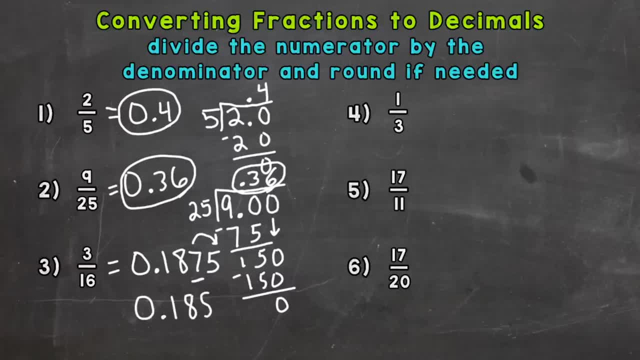 So our rounded answer would be one-hundred-eighty-eight thousandths. So that rounding step depends on what you're doing with the problem. Maybe you wouldn't round that decimal, depending on the situation, And as we'll see with number four and five, we can have decimals that are: 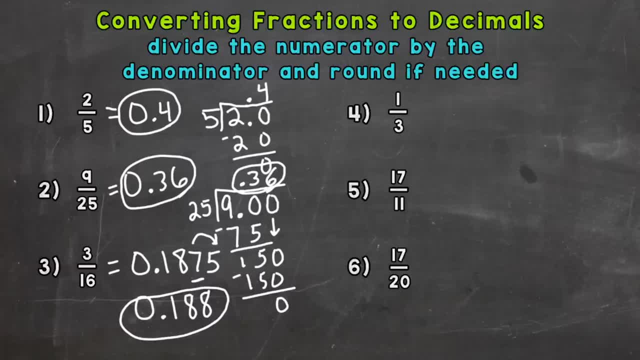 longer than just to the ten-thousandths place. So, speaking of number four, here we have one over three or one-third, And I'm going to show you this by hand and hopefully you'll notice a pattern as I start doing this. one, So one divided by three. So again, this is 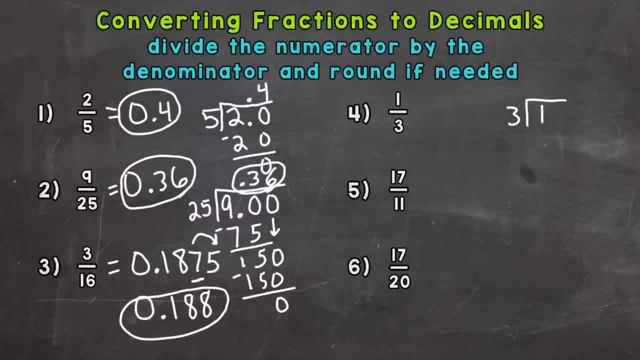 just like number one and two, where we wrote them out. We can't pull a whole three out of that one, We just need a decimal and a zero. Bring that decimal straight up, So we look at it as a ten. So how many whole threes can we pull out of ten? Well, three, That gets us to nine. Three. 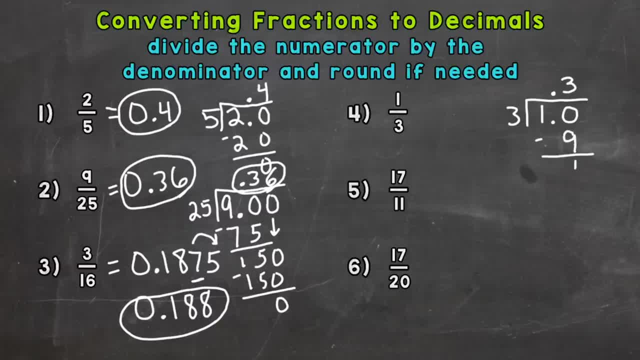 times three is nine. Subtract, we get one. Remember, we want that clean cut zero to tell us that we are done. So we need to add another zero. Drop it so we have another ten. How many whole threes out of ten? Well, 3.. 3 times 3 is 9, and our pattern is going to start here. Subtract add. 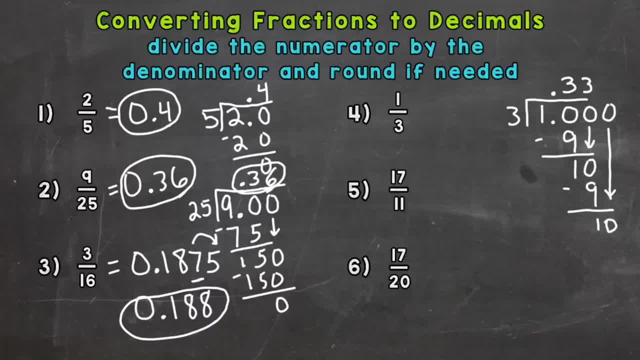 another 0 and drop it, so we have another 10.. 3 3's out of 10.. 3 times 3 is 9.. Subtract a 1, and you're probably getting the point here. It's going to go on. 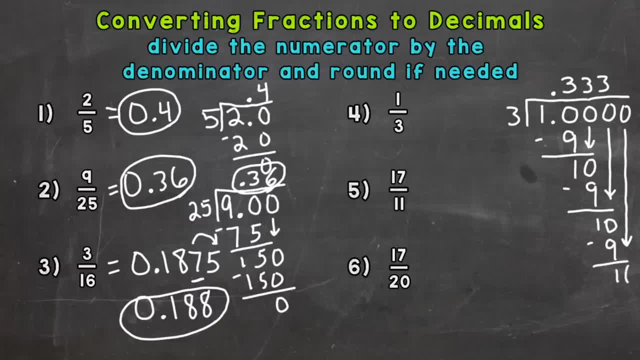 And you're probably getting the point here. It's going to go on forever, So it's a repeating decimal. So our answer This is one we would want to round And if we round it to the thousandths We have a 3 there. Look next door. It says: stay the same. 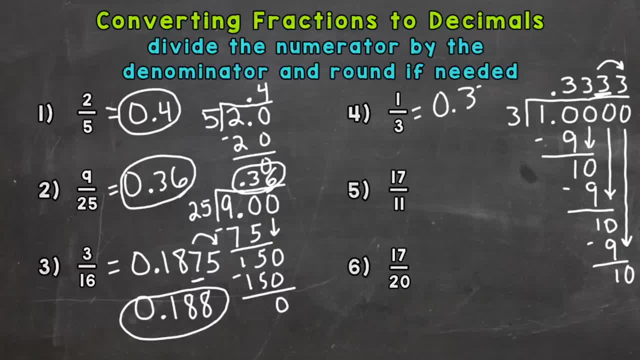 So our answer is 333 thousandths. Or if you have a repeating decimal, You can write whatever number is repeating And put a bar over it, And that bar signifies that that digit just repeats. Okay, So two ways to do that. You can round it off, Or the bar shows that that digit repeats. 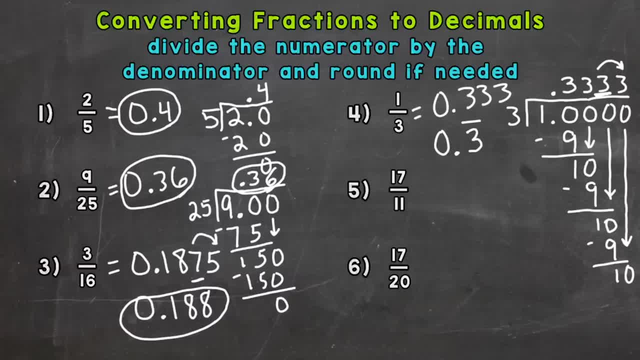 Or 5. We actually have an improper fraction, So this is going to be above one whole. It's greater than a whole. So if you plug 17 over 11. Or 17 divided by 11 in on a calculator, You're going to. 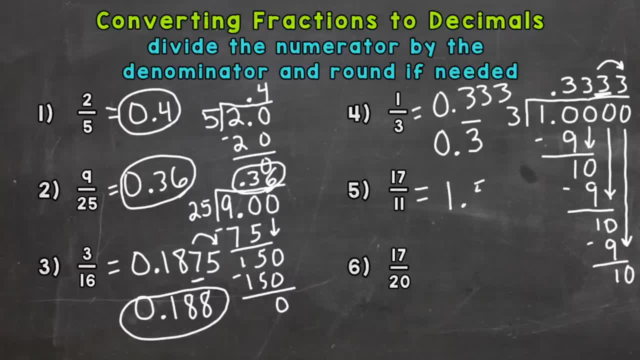 get 1.. 54., 54., 54. And it's just going to be 54's. repeating Again, we can round to the thousandths. So a 5 there. Look next door. That 4 says: stay the same. 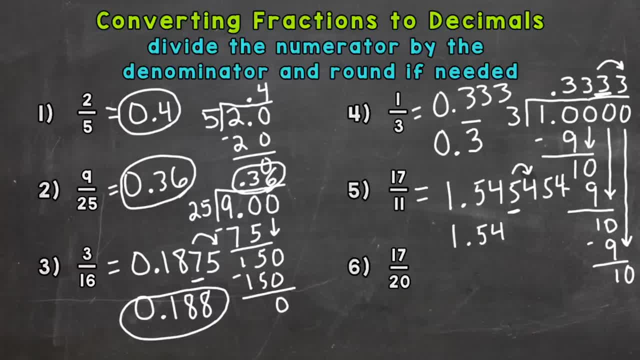 So our rounded answer would be 545 thousandths, So 1 and 545 thousandths. Or we can use the bar method- I forgot to circle my answers for number 4 there, Just notice that- Or we can use the bar method, So 1 and a 54 repeats, So we can put our bar above the 54 to show. 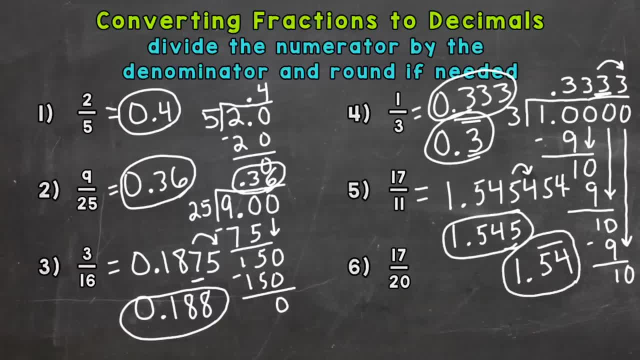 that that will continually repeat Number 6.. 17 over 20.. So 17 divided by 20 is going to give us 85 hundredths, So it cuts off in the hundredths place. So no need to round. That one works out. 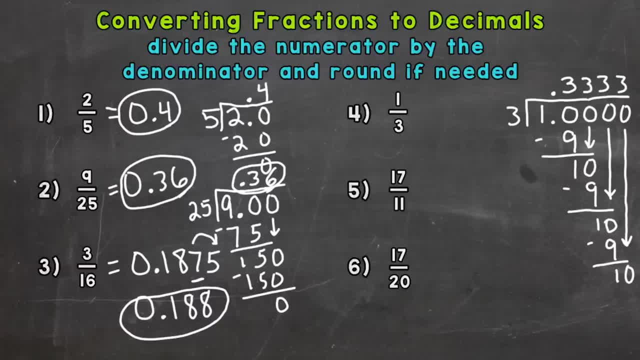 forever. so it's a repeating decimal. So our answer this is one we would want to round, and if we round it to the thousandths we have a 3 there. Look next store. It says stay the same. so our answer is 333 thousandths or. 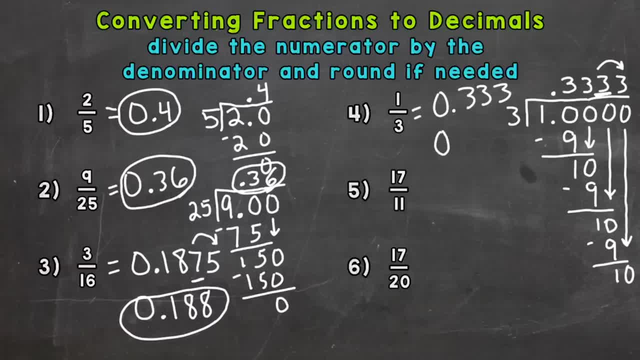 if you have a repeating decimal, you can write whatever number's repeating and put a bar over it and that bar signifies that that digit is a repeating decimal, just repeats. Okay, so two ways to do that. You can round it off, or the bar shows that that digit. 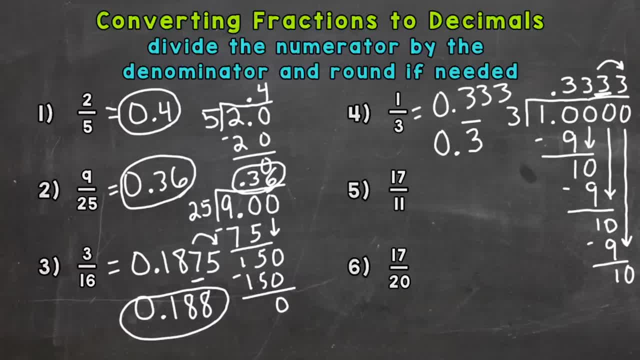 repeats. So number five: we actually have an improper fraction, So this is going to be above one whole. It's greater than a whole. So if you plug 17 over 11 or 17 divided by 11 in on a calculator, you're going to get 1545454.. And it's just going to be 54s repeating. So again, we can. 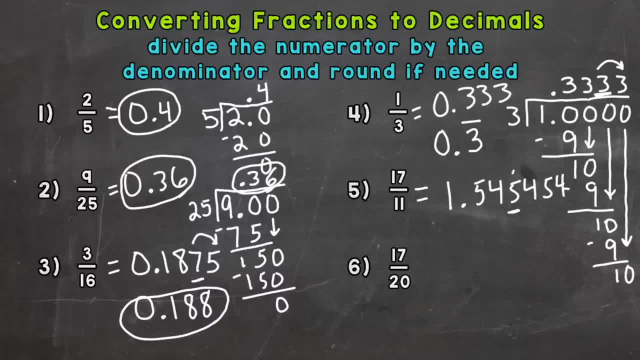 round to the thousandths, So a five there. look, look next door That says that four says stay the same. So our rounded answer would be 545.. Thousandths So one and 545 thousandths. Or we can use the bar method. I forgot to circle my. 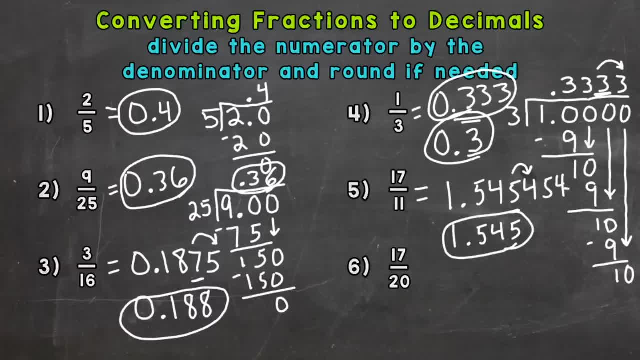 answers for number four there Just notice that: Or we can use the bar method So one and a 54 repeats, So we can put our bar above the 54 to show that that will continually repeat Number six: 17 over 12.. 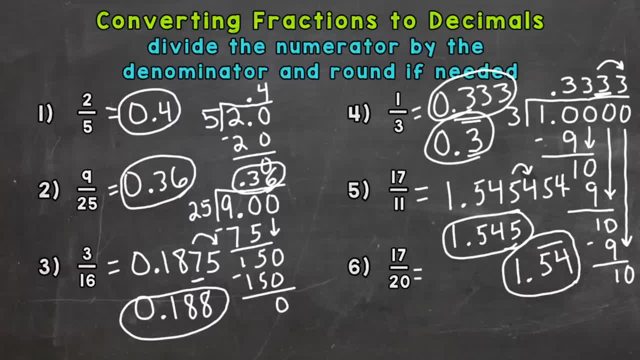 So 17 divided by 20 is going to give us 85 hundredths, So it cuts off in the hundredths place. So no need to round. That one works out nicely. So there you have it. There's how you convert a fraction to a decimal. Divide the numerator by the denominator and then interpret.